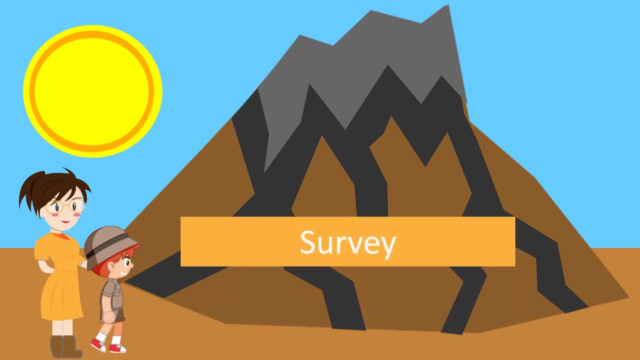 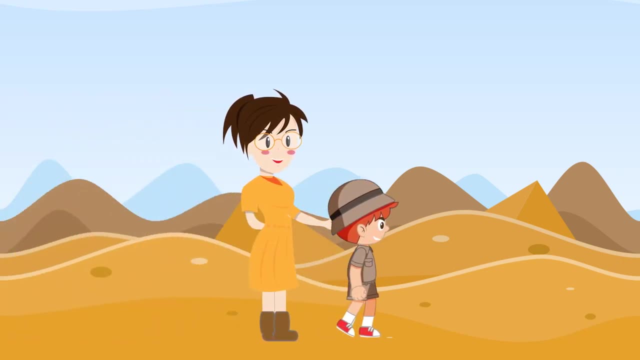 Jacob doesn't do much digging, but the last few days he has helped his mom with a survey. Today they are in the New Mexico desert, not far from the Rio Grande River, working on a site survey of an old campsite on one of the oldest trails in North America. 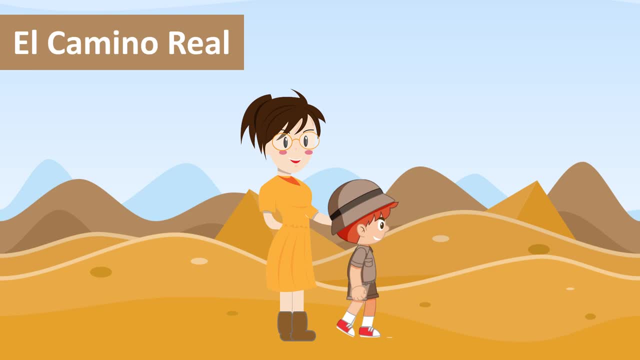 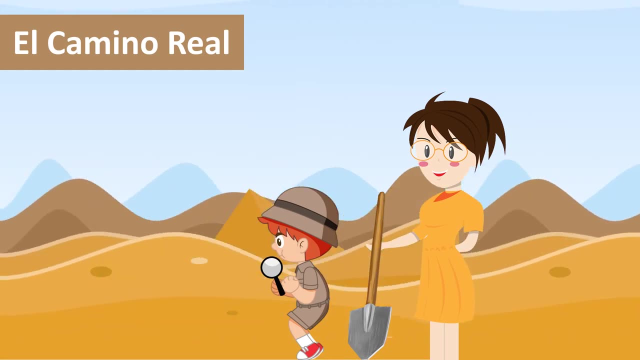 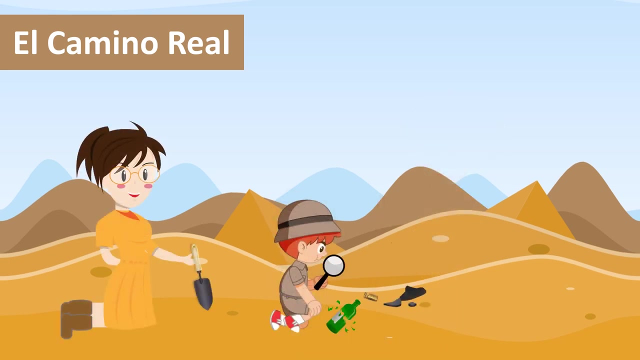 El Camino Real. For over 400 years, people have traveled this 1,600 mile route. Jacob is looking for old objects visible on the surface of the ground while his mom digs for them. Yesterday they found pieces of broken ceramic bowls from the 1600s, pieces of glass bottles and even some old ammunition scattered all over the site. 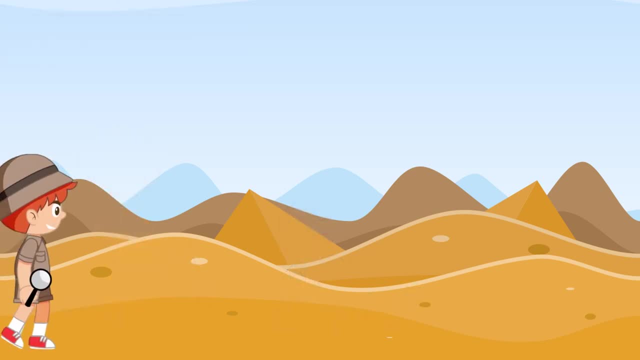 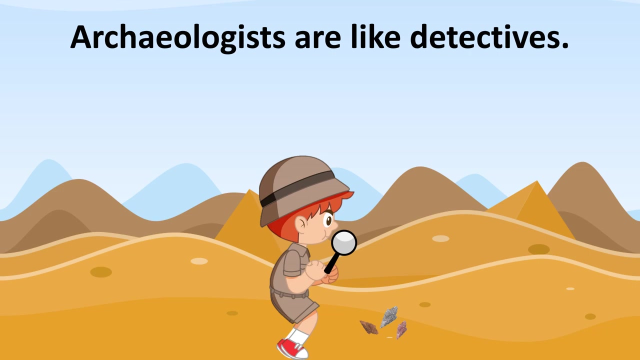 And they didn't even have to dig. No one knew what they would find today, but Jacob knew it would be interesting. He was ready to go. What is an archaeologist? Archaeologists are like detectives: They study human life by looking at artifacts, which are the man-made objects the people who lived long ago left behind. 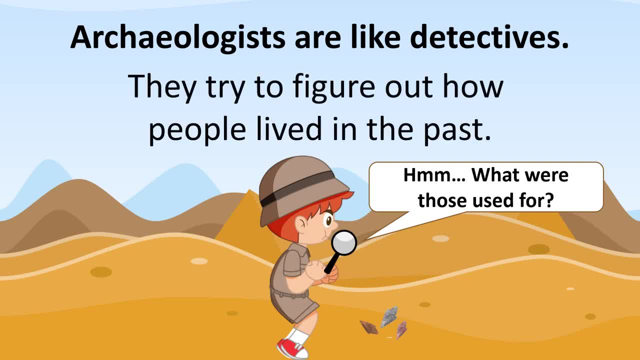 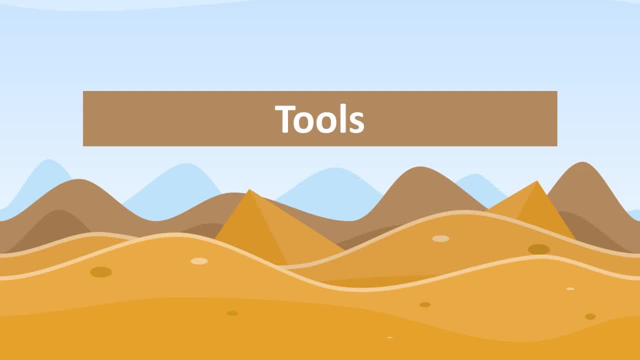 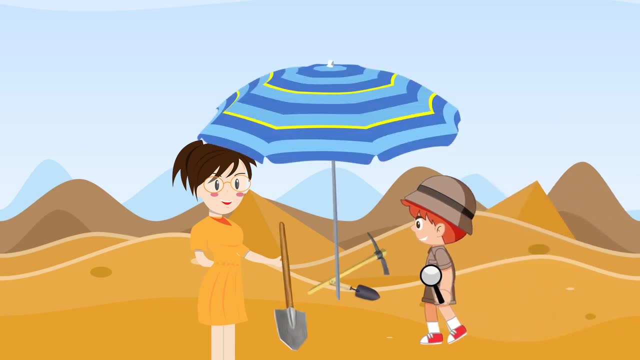 By looking at objects, they try to figure out how people lived in the past. Tools of an archaeologist: Archaeologists have a wide variety of tools in order to do their job and to find artifacts. Jacob took some of those tools on the dig with his mom. 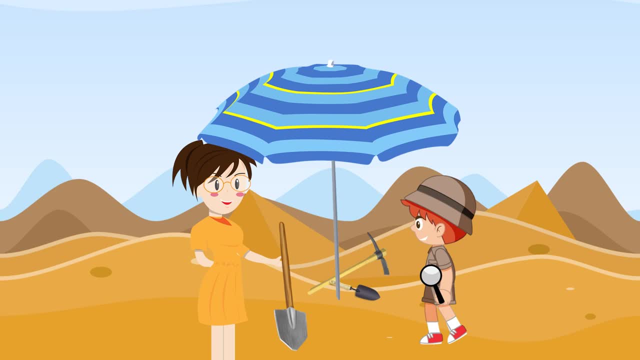 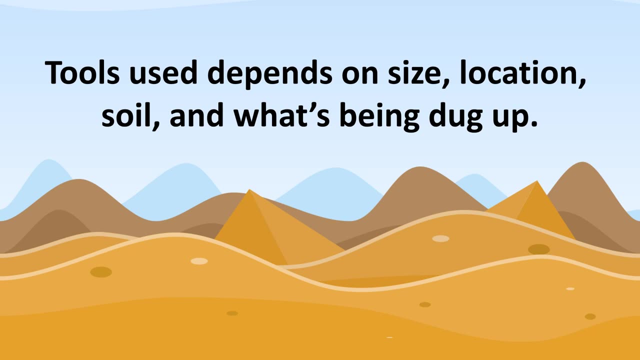 Some of these tools are very specialized and expensive, and some are common and cheap. to get Exactly what tools are used depends on the size, location and type of soil at each site and what is being dug up. These tools can include screens. 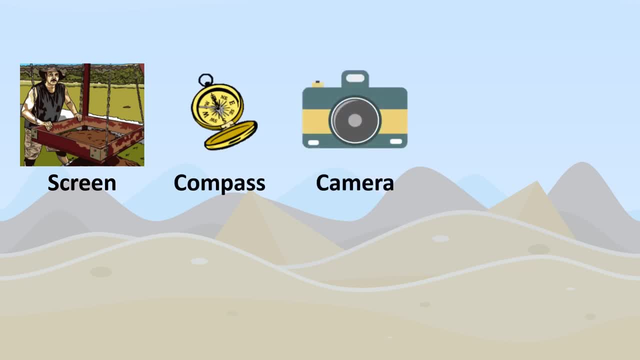 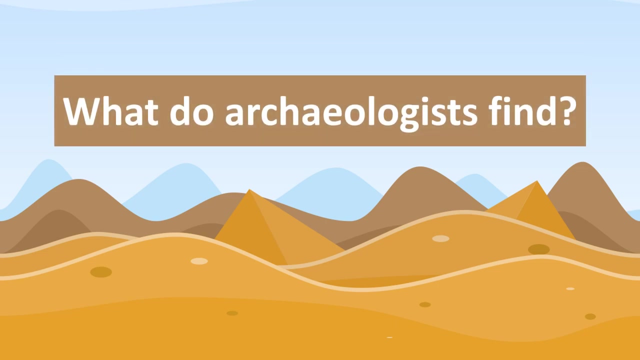 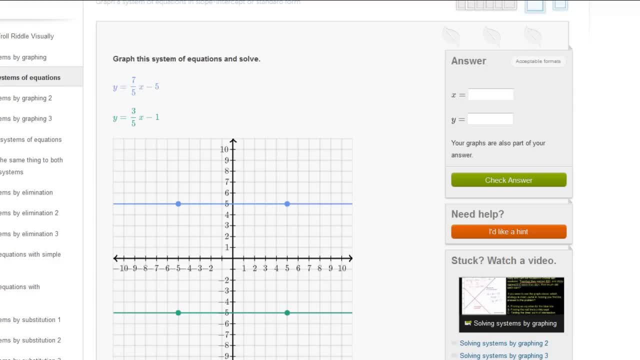 Just in case we encounter any more trolls who want us to figure out what types of money they have in their pockets, we have devised an exercise for you to practice with, And this is to solve systems of equations visually. So they say, right over here, graph this system of equations and solve. 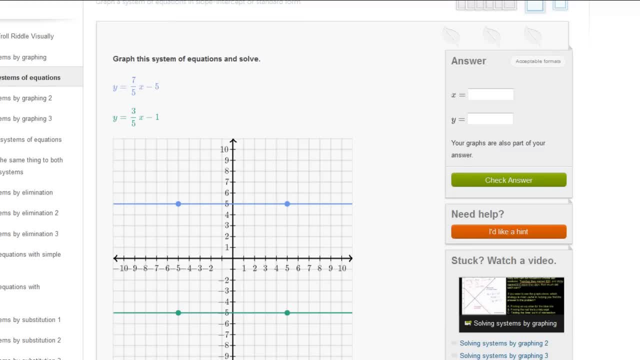 And they give us two equations. This first one, in blue y, is equal to 7 fifths x minus 5.. And then this one in green y, is equal to 3 fifths x minus 1.. So let's graph each of these and we'll do it in the corresponding color. 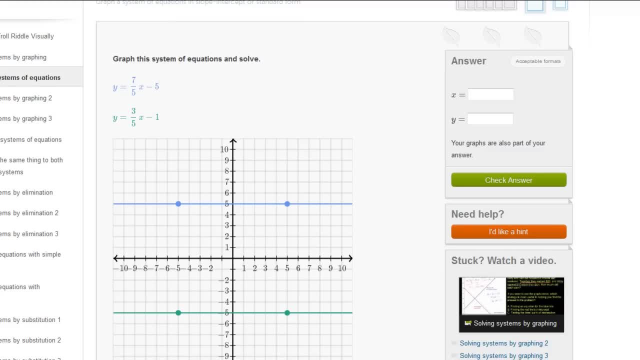 So first let's graph this first equation. So the first thing I see is that its y-intercept is negative 5.. Or another way to think about it: when x is equal to 0, y is going to be negative 5.. 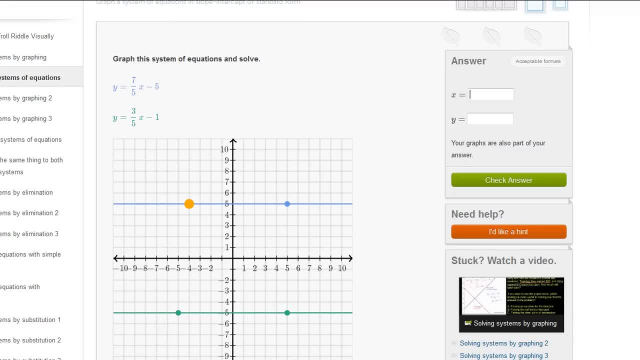 So let's try this out. So when x is equal to 0, y is going to be equal to negative 5. So that makes sense. And then we see its slope is 7 fifths, Which was conveniently placed in slope-intercept form for us.